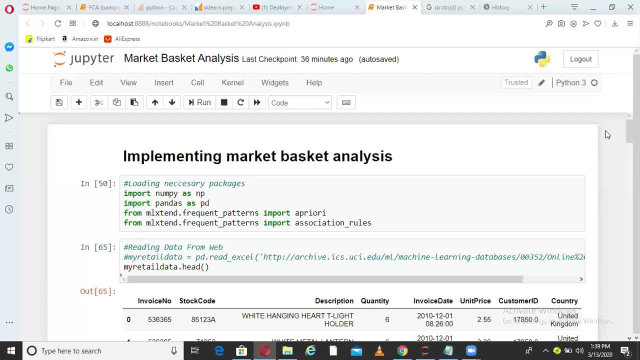 transaction. we know that people who buy chips packet are likely to buy a mayonnaise or sauce or those kinds of stuff. So maybe somebody who buys a chips packet, we can recommend them a mayonnaise or sauce or things like that. So how to implement that particular thing in Python? 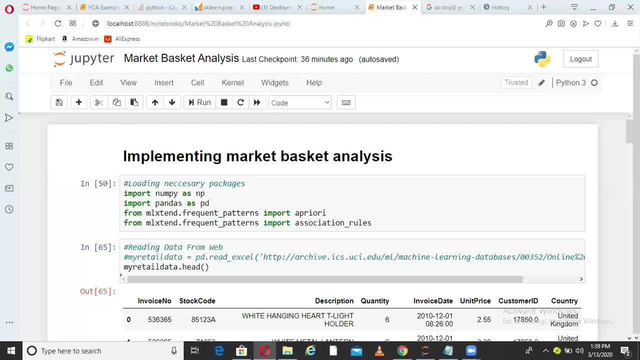 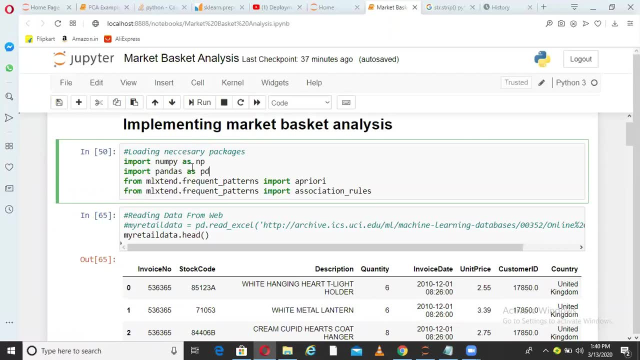 Let's see here step by step. Okay, So in the very first block, what I'm doing here is I'm trying to import some of the packages that I will need. These packages are numpy pandas, And two important packages here are ml, extend, dot, frequent patterns. So this is one package if you do not have in your 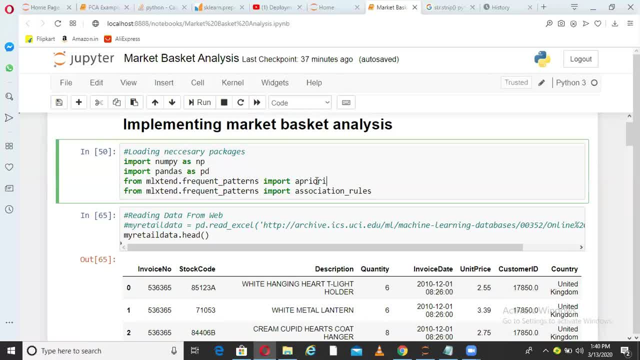 Python. right now you need to install this. Okay, So I'm importing a priority from this particular package, And other package which I'm importing is association rules from ml extend dot frequent patterns. So this is another package that you need to install in Anaconda. 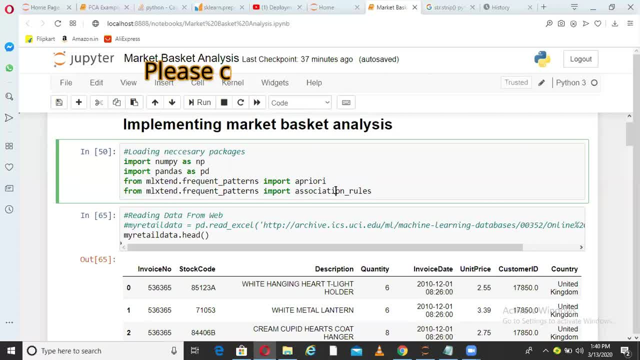 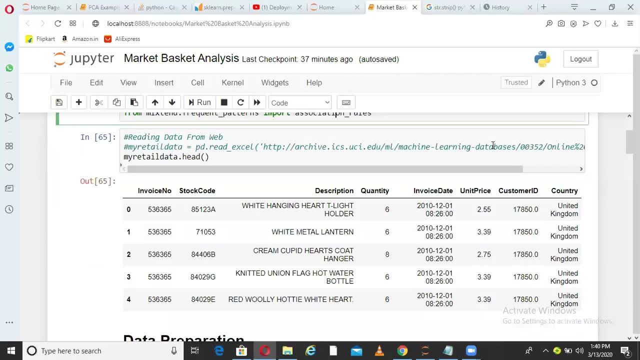 If you do not have this package with you. Okay, So this is the package we will use in this analysis or in this implementation. Okay, Moving forward, what I'm doing in next step is I'm reading a file from this particular location. So what is this location is? there is an Excel file in this. 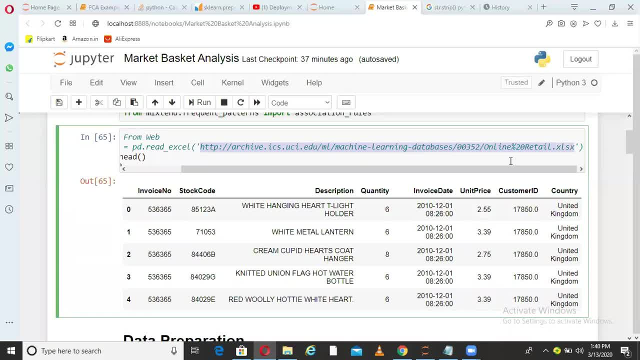 location If you go to this particular URL. in this URL I have an online retail data. Okay, That particular retail data, that particular transaction data, I'm reading using pd dot, read underscore: Excel: Okay, And I'm calling that data frame as my. 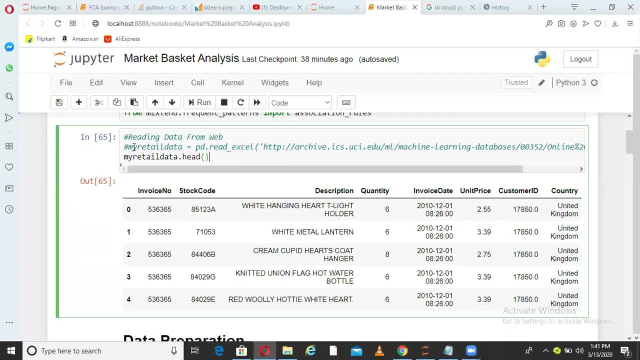 retail data. So I have knowingly commented this line because it will take some time to read. Now I have already read this data And, if I run this, as you can see, this is how this data looks like. Okay, So this data is basically an online retail data where we have 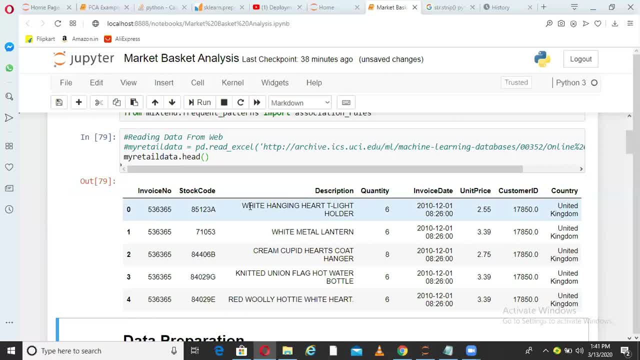 an invoice number, we have the stock code, we have the description of the product, we have the quantity, we have the date of the invoice, unit, price, Customer ID and country. So this is how this online retail data is looking like. Now we will. 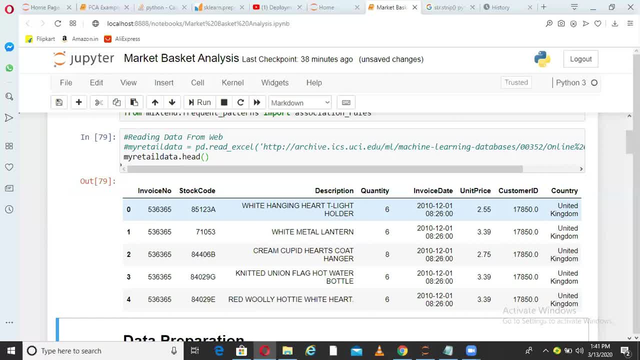 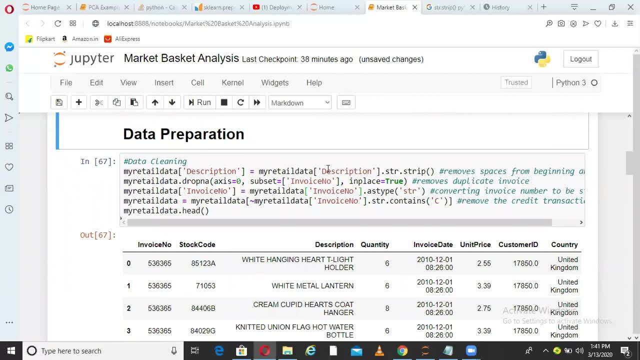 run association analysis on this particular data. Okay, Moving forward, I'm doing some data preparation here. So very first thing I'm doing here is I'm just removing the space from the description column. As you can see, description column has, you know, some characters of some. 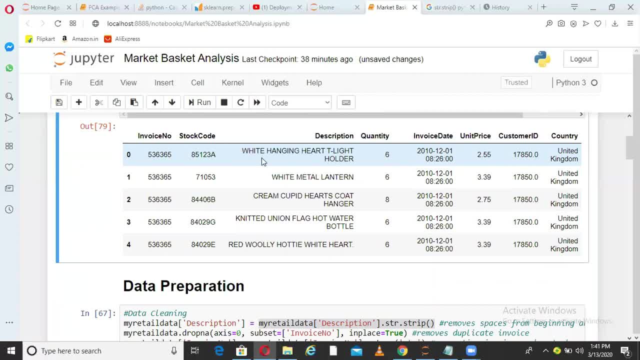 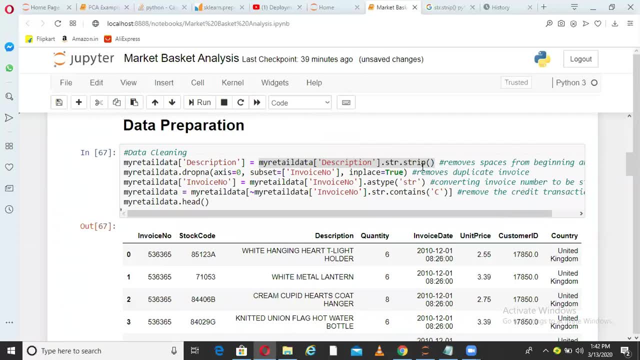 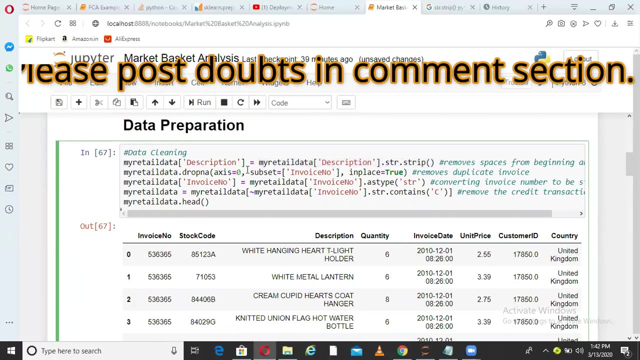 sentence kind of thing. So there is a possibility that there might be spaces here before the sentence And after the sentence. So that is what I'm doing in this line. I'm just removing the space, Okay, So that only the product description is there. I'm also subsetting the invoice. 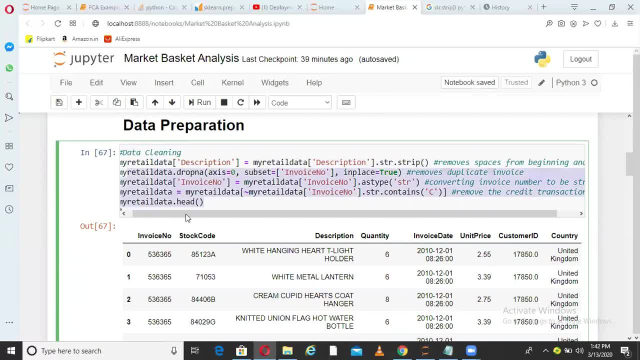 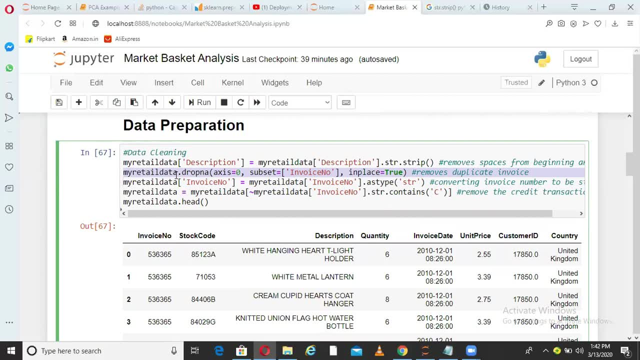 and I'm dropping all the NAs from the invoice. So if, if there are any invoices- where there is any, if there are no invoice number, then I'm removing those records. Okay, And also what I'm doing here is I'm just converting the invoice number to type. 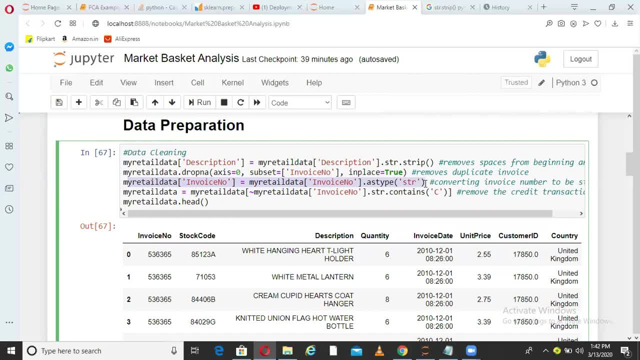 String. This is needed because when we run, the analysis algorithm understands the invoice number as a string data type. Okay, In the next line, what I'm doing here is I'm just removing the credit type of invoice. So how do I know it's a credit type of invoices? 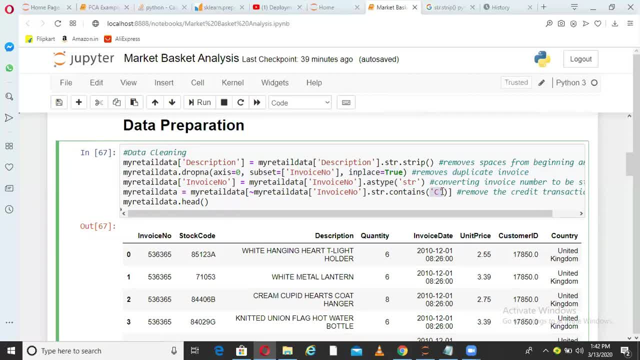 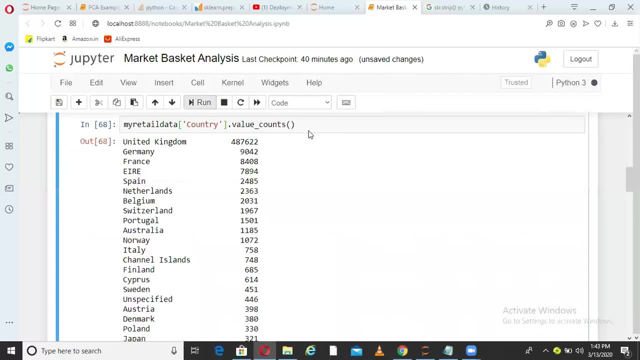 I just see a particular keyword or a particular alphabet C, and then they come to know that that is credit invoice And hence from my analysis for now I'm removing those credit saya Iftee credit invoices, invoices. after doing all this cleaning, data cleaning- what i have is the clean data with me. 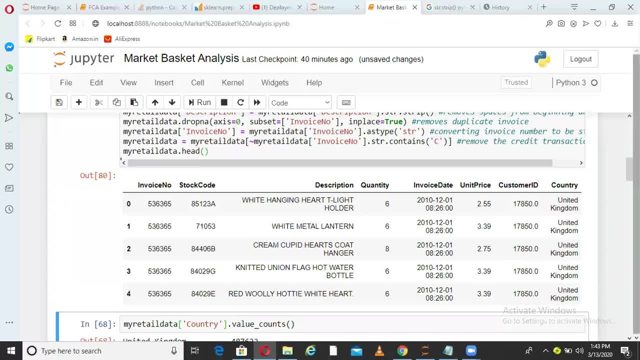 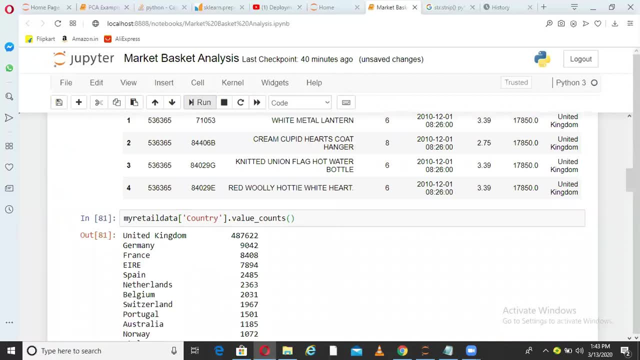 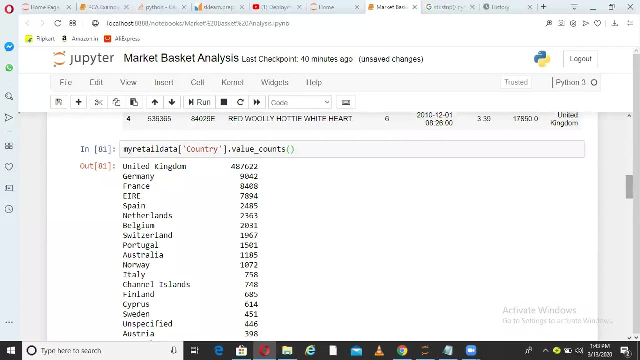 which looks like this. okay, from this clean data, what i'm seeing here is: what is the value count or what is the record count for different countries? as you can see, the last column here is country, so i just want to see which country has how many records. okay, so united kingdom has. 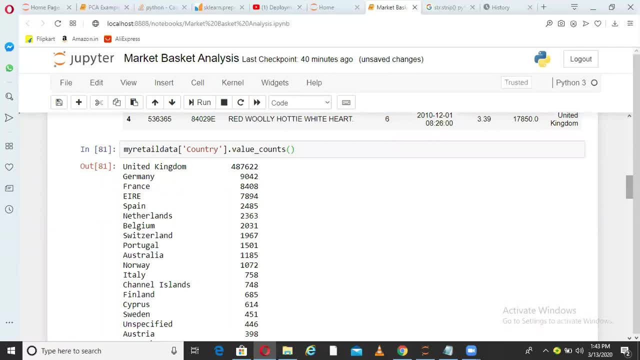 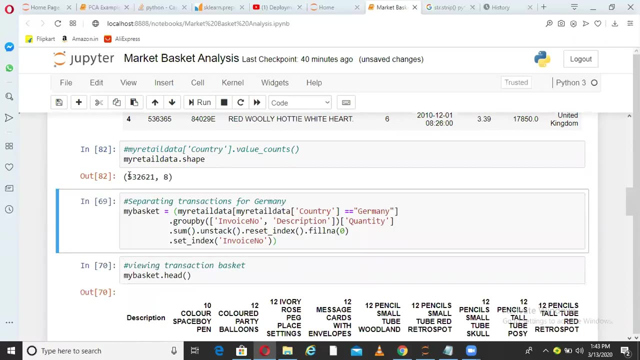 highest, then comes germany, then comes france. so the size of the data is too much. so let me check what is the size of the data here. so if i say my retail data dollar shape, it should give me the size of my data, okay. so the size of my data is 532k, which means 532k records in my data. 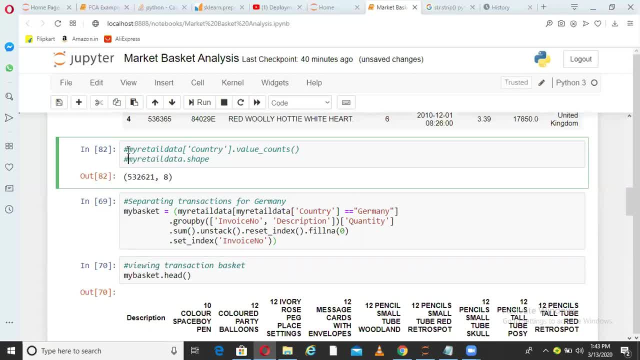 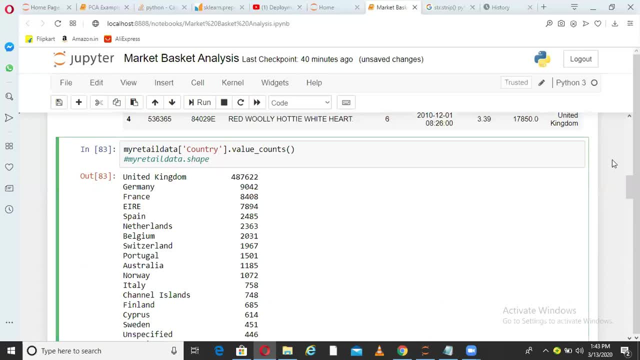 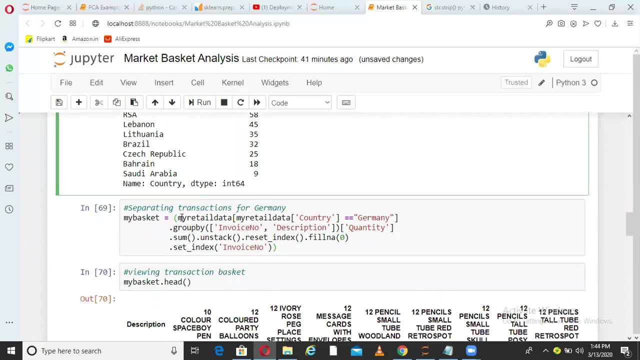 out of those 532k records, as you can see when i run value counts, 487k is uk records only and rest are other countries. so what i'm doing in the next step is i'm just filtering the data on one country. if you can see, here i'm saying my retail data country is equal to germany, so why i'm? 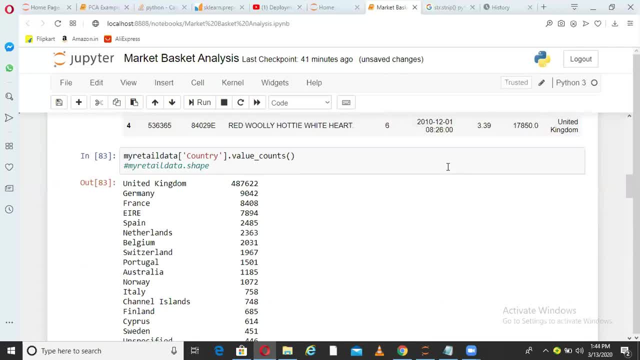 doing, that is, i do not want to run the analysis for all 550k transactions, close to 550k transactions. what i want to do is i want my analysis to run faster for demonstration purpose, and hence i'm running on country germany only okay. so what i do here is: 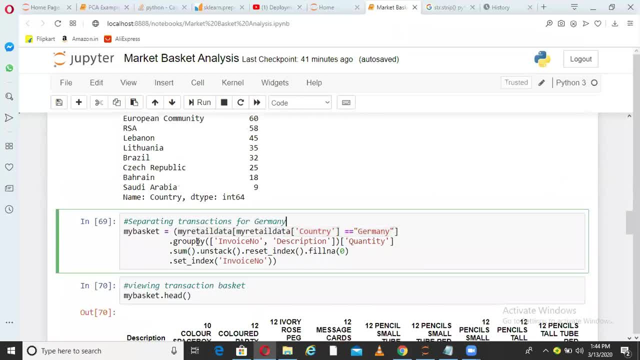 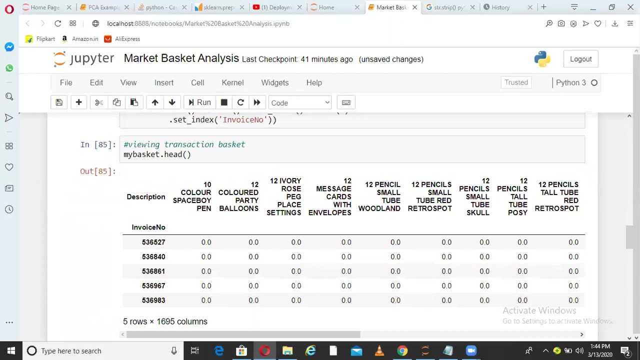 i take all the transaction of germany, then i group by on invoice number and description and i just take a sum of the quantity. so what this entire code will do is it will give me a basket of transactions. so how that basket of transaction will look like is this so this invoice number? so 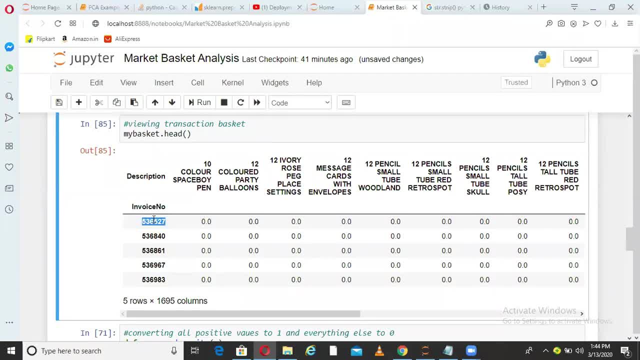 from the main data, from this, from the excel file that we have imported. now i have a basket data. i'm calling that my basket. so how that basket data looks like. it will have a invoice number as key and these are the name of the products: 10 color space boy. 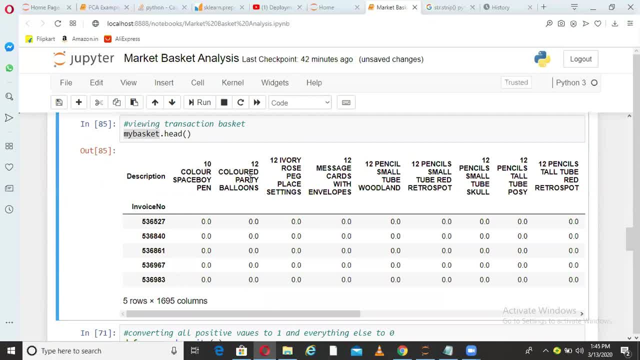 pen, 10 colored party balloons. all these things are name of the products. so if the value here is zero, that means that product was not not present in this invoice. and if we have a positive number here, for example one, two, three, four, five, six, anything that means that product was a part of. 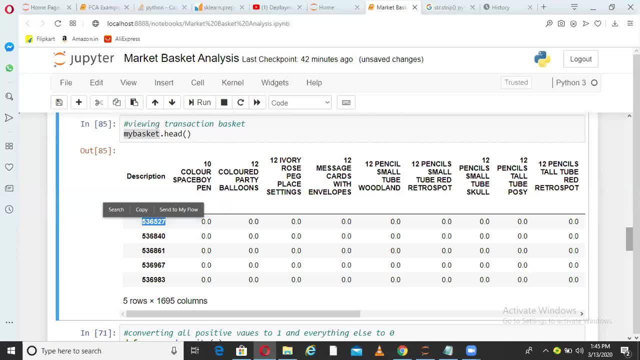 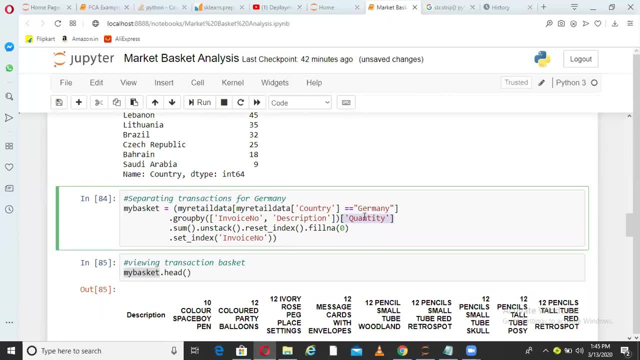 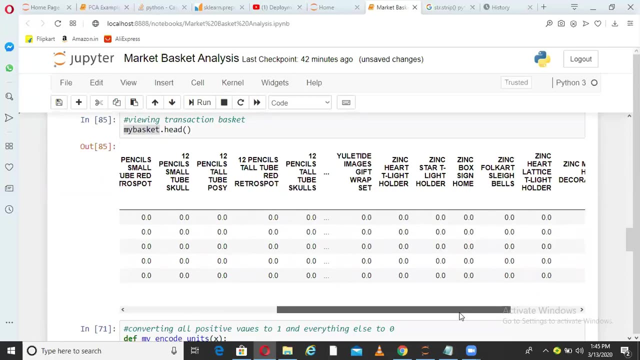 this inverse those many times. as you can see here the sum is done on the quantity. so i'm saying group by on inverse, number and description and sum on quantity. so what we will see here: all the records are not getting displayed. if we export it to csv and c, we will see some. 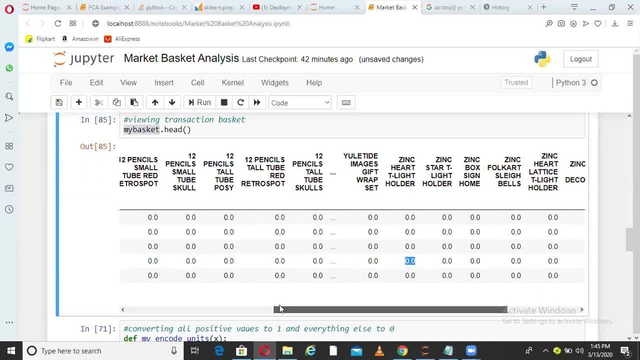 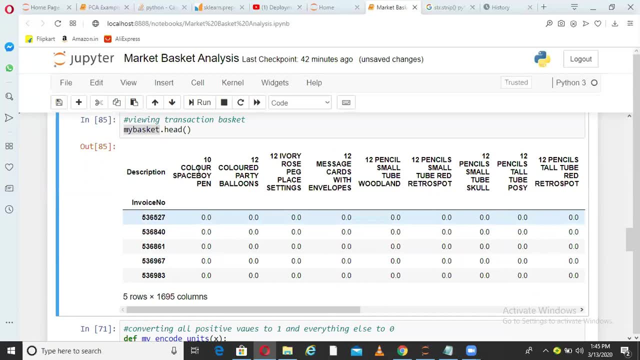 numbers here. some values will be zero and some values will be numbers. numbers means those particular products are part of that inverse. okay, and zero means this particular product is not the part of this inverse. that is what i'm doing. i'm just creating a basket of transactions. 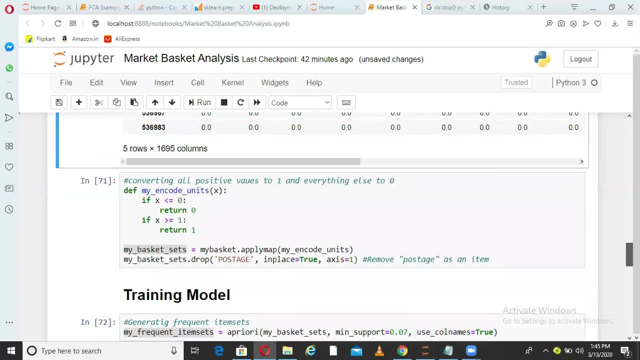 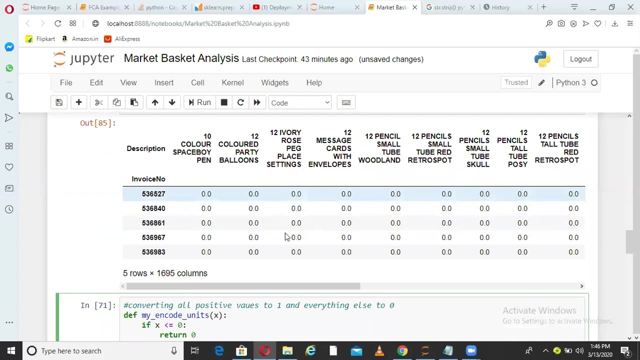 i'm just creating a basket of transactions, so this is going to be the first step. moving on to the next step, what i'm doing here is i am just defining a small function which converts all zero, all the numbers which are less than 0 to 0 and all the numbers which are greater than 1 to 1. 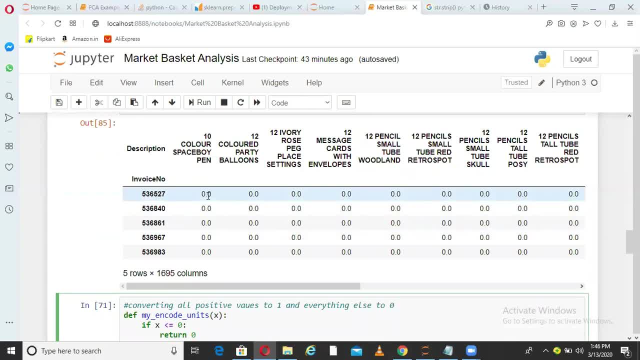 so why i'm doing that is, i want this data frame or this data to become only 0 and 1, because that is what my algorithm expects as input. okay, so all these zeros will remain zero, but there will be numbers, for example, one, two, three, four, five, So all those numbers will be converted. 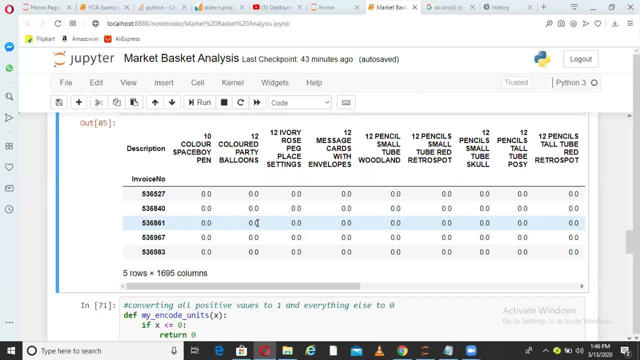 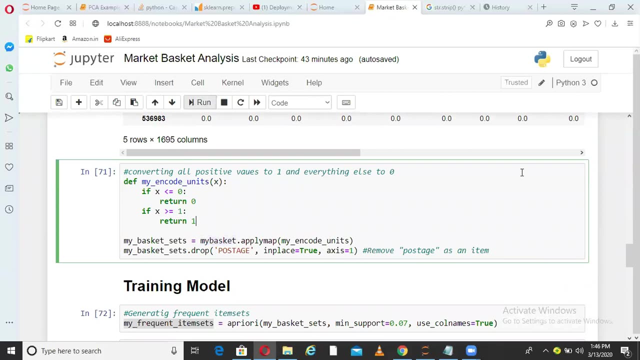 to one. Why I'm doing this is: this is how the algorithm of association analysis expects the input data to be in the form of zero and one. Okay, So I learn this function on this particular data or this particular basket. So what I will have? I will have all these. 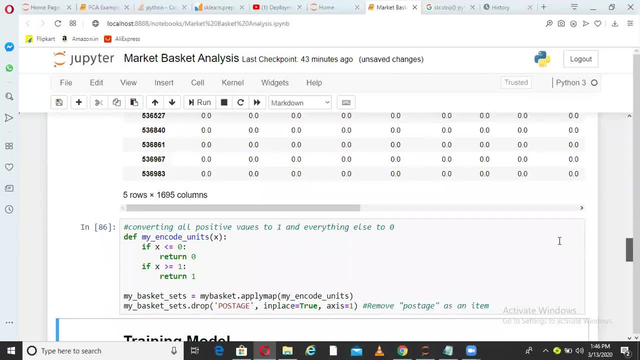 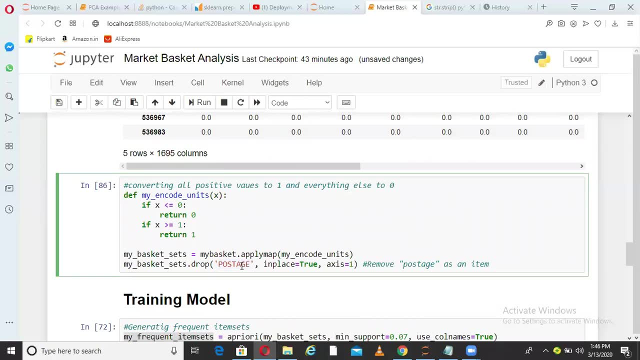 zeros and ones in this data. now, Okay, And there is a postage column which is not needed, postage, you know, item which is, I think, does not make much sense. Hence, I am removing that postage column from the data, from this, my basket, Okay. Coming to training the model. 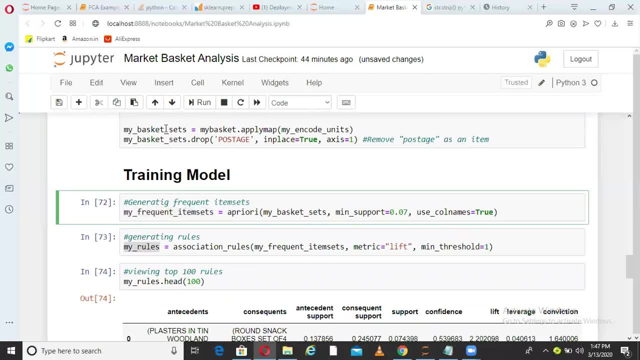 how do we train the model? So now we have my basket sets, which means my basket transactions, after the above data conversion zero and one encoding conversion. Okay, So what I'm doing here is I'm just running a priority on my basket sets, Okay, So where from a priority? 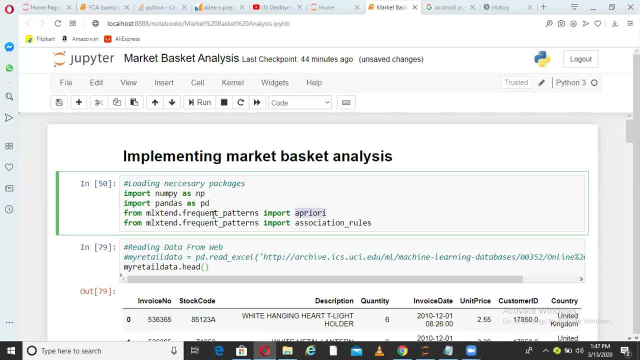 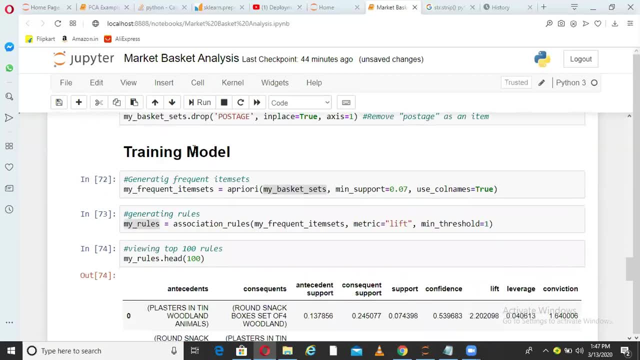 is coming. You see, here I have imported from ML extended frequent patterns, Okay, So what I'm saying here is I'm saying here a priority. my basket sets. my basket sets is just now I've created. minimum support is equal to zero point five. So in my last video I had explained what is lift. 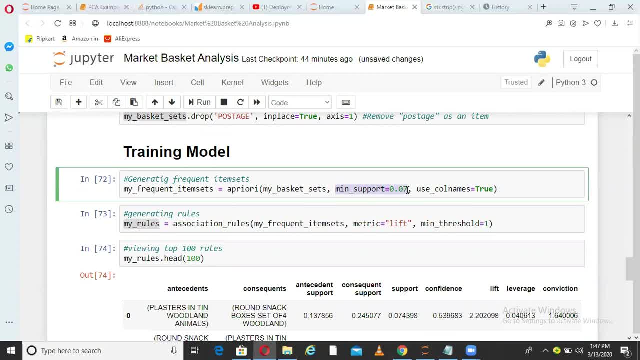 support and confidence. So that is what defines the goodness of your rule or the strength of your rule in association analysis. Okay, So I'm saying minimum support is equal to zero point zero seven, which means: consider the rules. which has this much of support? 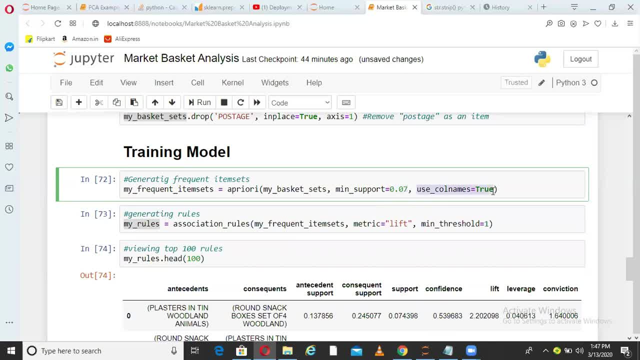 and use column names is equal to true. that means use my column names as item names. okay, how do i generate rule from my frequent item sets? so what this will give is: this will give me the frequent item sets. okay means kind of transactions. how do i generate rule from those transactions? 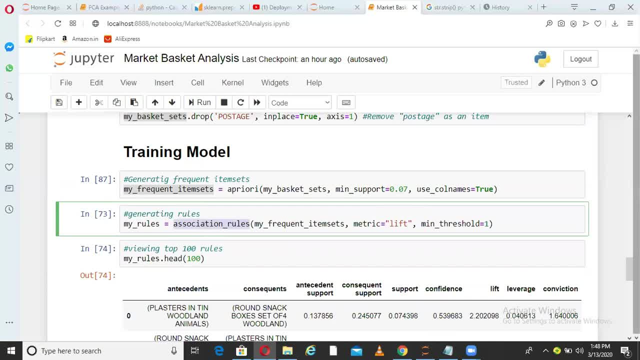 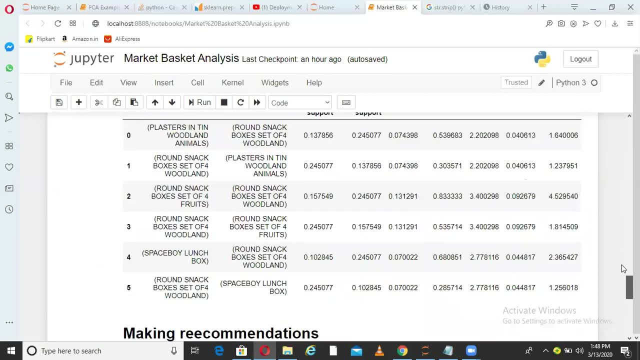 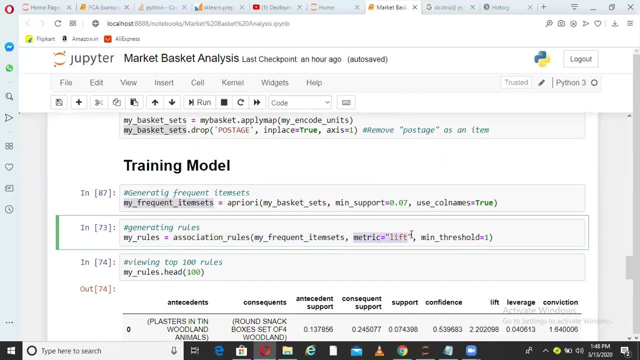 so i just say: association rules, where from association rules is coming from here, ml extend or frequent pattern association rules? so i am just taking the association rules, giving my frequent atom set as input and saying: take the metric as lift. so out of support, lift and confidence, take the metric as lift and put the minimum threshold as one and then give me the. 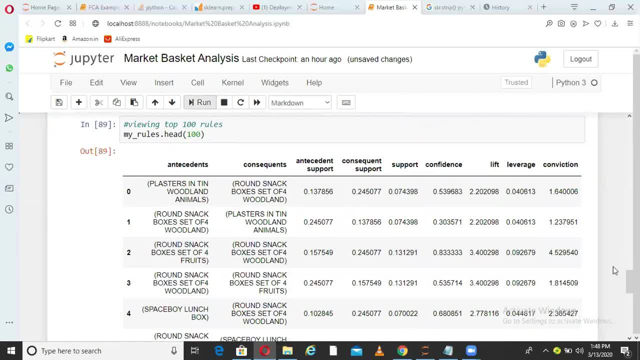 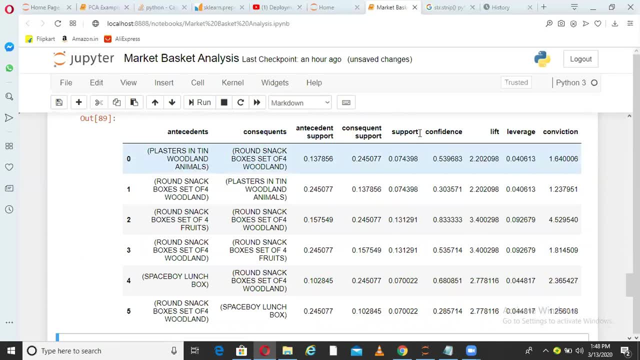 rules. okay, once i run that, this is how my rules will look like now. this is important to understand, guys. in my last video i explained you about support lift and confidence okay, and i had told you there will be item a implies item b with a particular number of support lift. 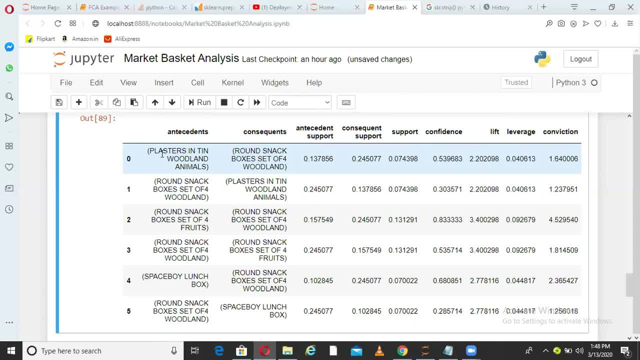 and confidence, and that is what you can see right here on the screen. so plastic in tin, woodland animals- this is one product, product a. product a implies product b. so what is product b? product b is round snake box set up for woodland. product a implies product b. the support is 0.07. the 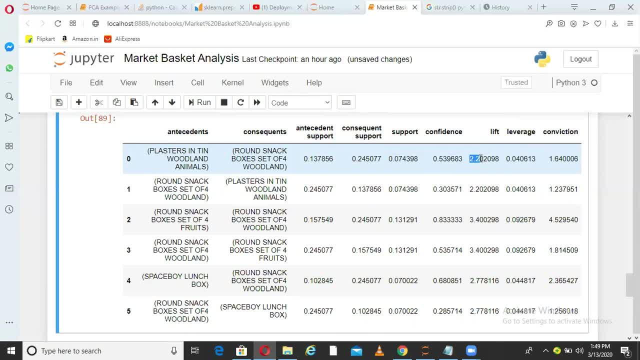 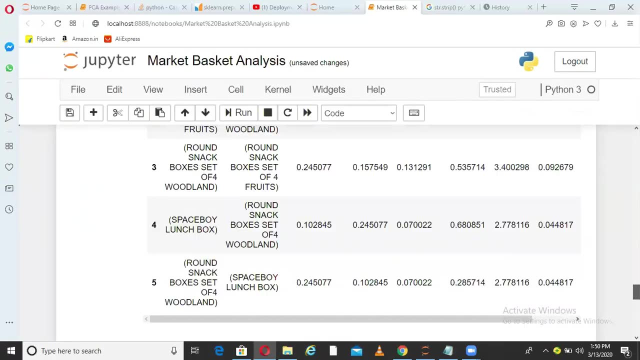 confidence is 0.53 and lift is 2.2. okay, and similarly, product a to product b will have different, different support, lift and confidence for different, different combination of products. now how do we use these rules to make recommendation? let us see here, coming to rule number five. so this is the rule table which you can see here. 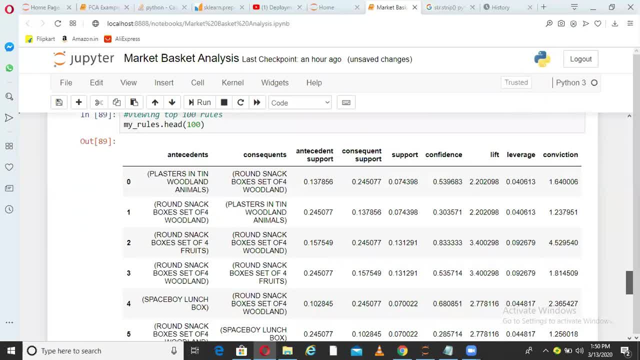 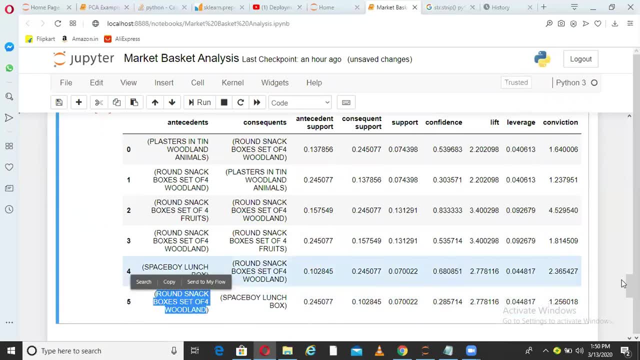 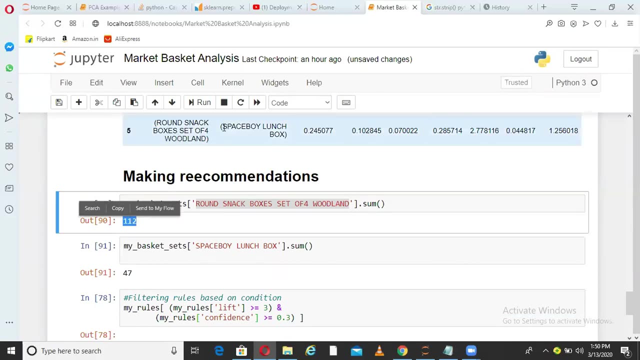 coming to rule number five from the rule table. so this is the rule table from my rules. if we see rule number five, the item a is round snake box set of four woodland. okay, so how many times this is occurring? one, one, two times. the item b is space for lunch box. how many times this is occurring? 47 times, which. 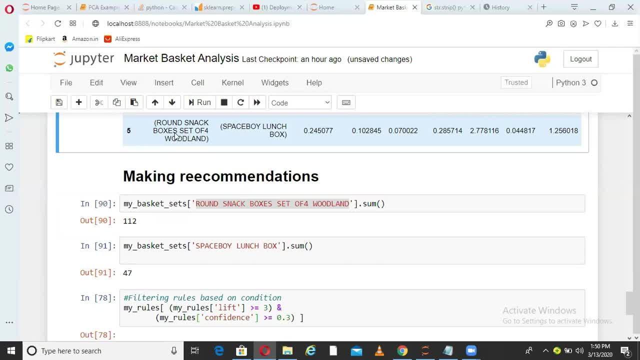 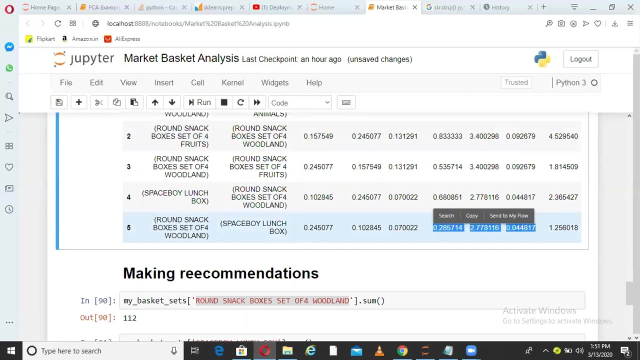 means that people who are buying one, one, two times item a out of those, only 47 times item b is being bought. but the set of rules says that there is a good support, lift and confidence for this combination, which means that we can recommend item b, which is specific space for lunch box to. 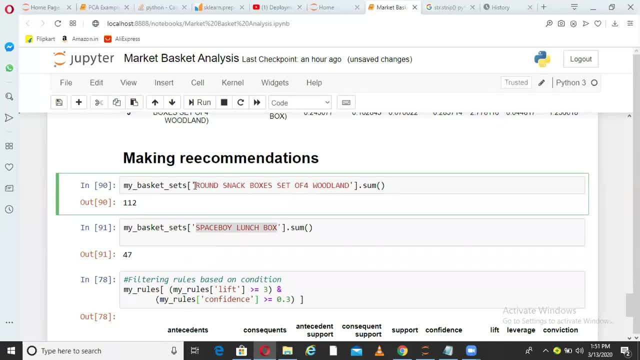 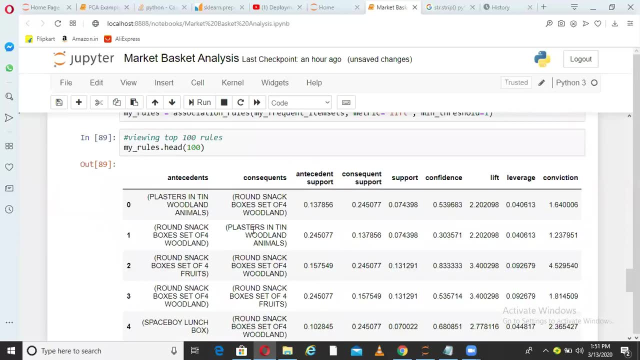 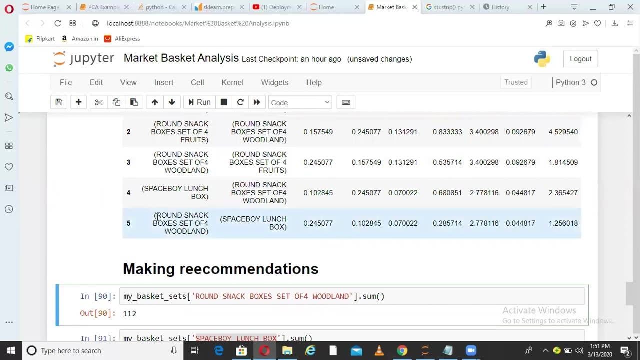 some one who is buying round snake boxes set of four woodland, okay. so i'm repeating it again: rules are giving us different rules, so here i am printing different rules from the appaready algorithm. out of those rules, i consider one rule, rule number five. in this rule number five, i see: 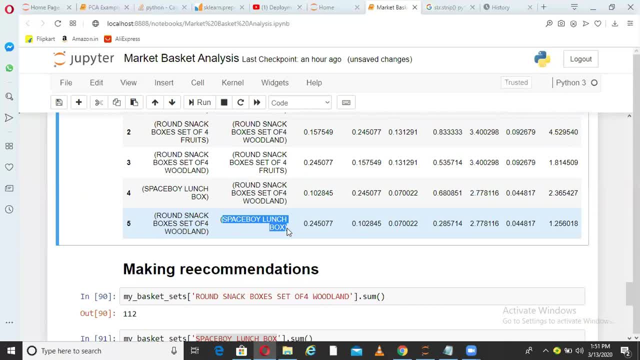 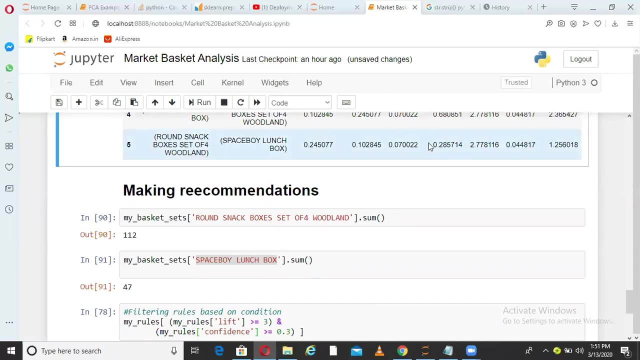 two items, item a and item b. i see how many times item a are present in the transaction one, one, two times how many times item b is present independently in the transaction one. so i'muga case one, two, three, four, seven times. but we see a good support, lift and confidence. 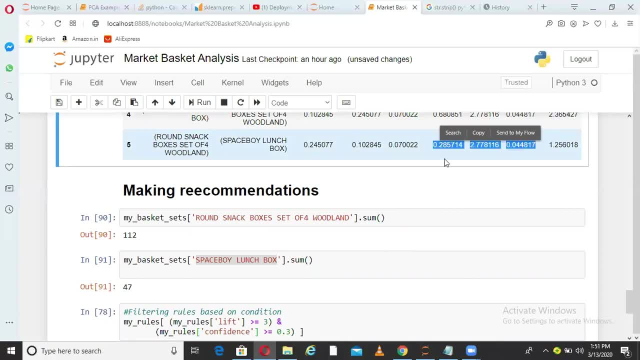 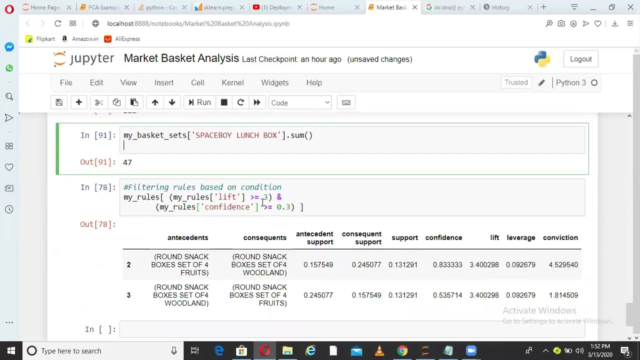 number here for these two items, which means that every time this product is bought, we can recommend product b as well. okay, and that is how the recommendation can happen. also, we can also filter on what support, lift and confidence we want, our rules, for example. here i'm saying: 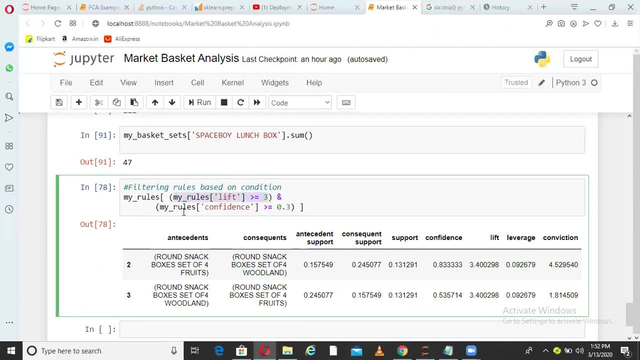 give me the rules where lift is greater than 3 and give me the rules where confidence is greater than 0.3. so I am just limiting my rules to only two rules as of now. so these two rules will have these two characteristics of these two. 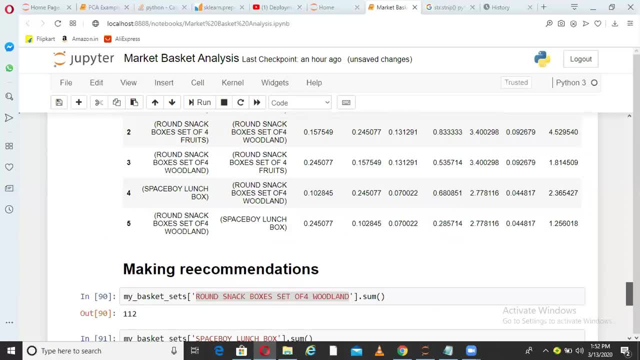 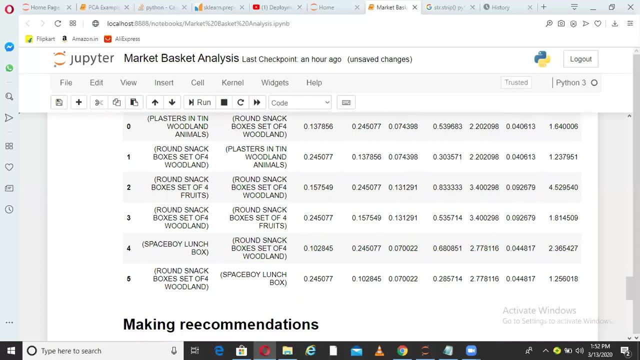 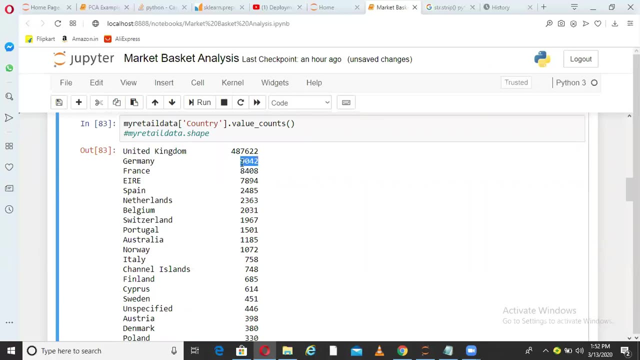 filters. similarly, we can go on and compute more rules, get more rules from the transaction. so how many rules we will get, it totally depends on what is the volume of transaction we are giving here. so if you see, here in Germany we have only nine zero four, two records, which means nine zero four, two invoices. 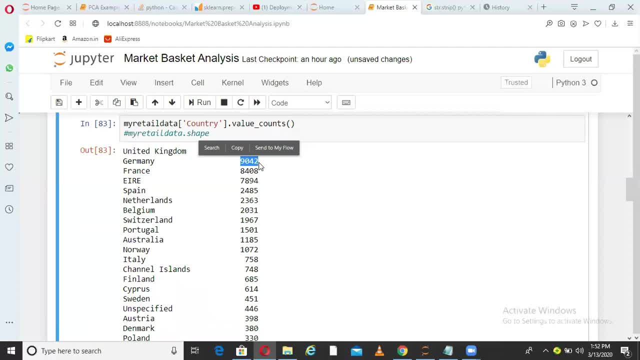 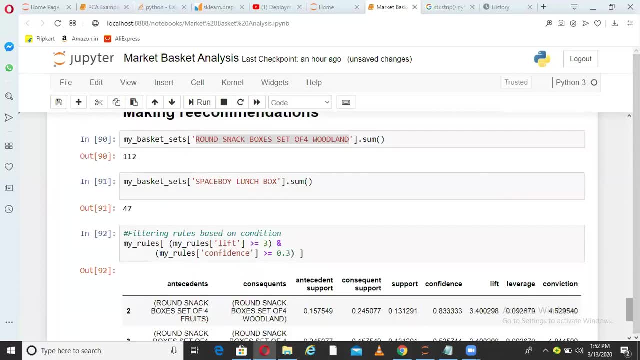 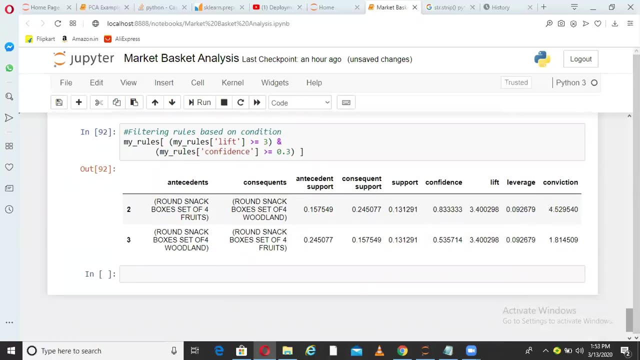 so, out of those nine zero four, two records or you know, transactions, we are getting these many rules. if we give more transactions, we will get more rules and more strong rules. so this is how, using the transaction, you can create rules and those rules you can use to make some recommendations based on support lift. 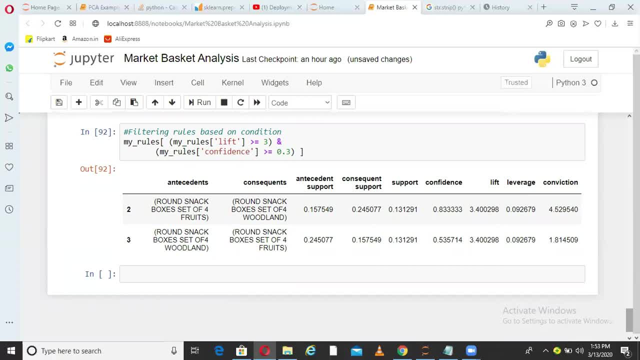 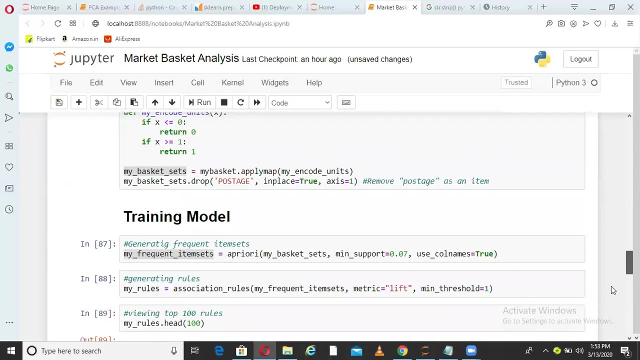 and confidence, and this is one of the very basic and common recommendation process used in detail scenario known as association analysis or market basket analysis. so I have kept this very simple, knowingly, so that you can grasp the concept. there are other things also in the output, for example leverage or conviction. all these things are just interrelated to support. 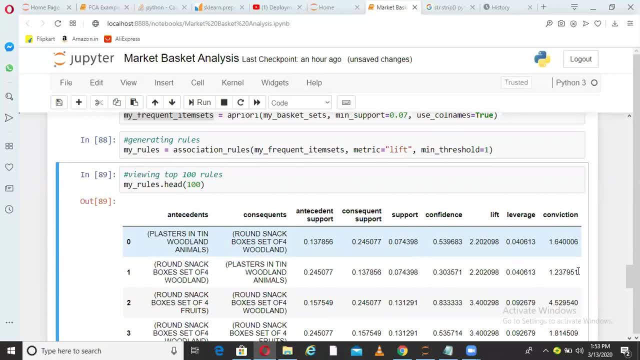 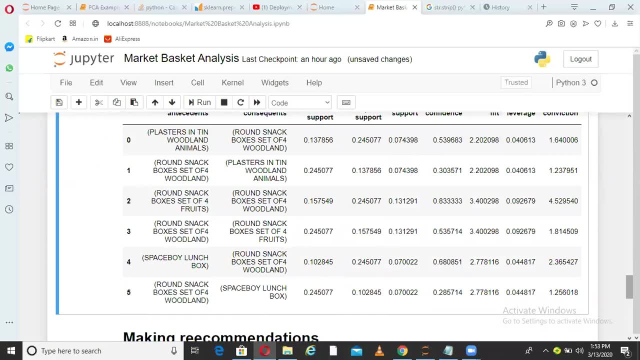 lift and confidence. you can just go ahead and learn about these things as well, but more important things here are support, lift and confidence, and this is on what we put threshold, on what we put threshold on this and this will be our sold and we give the recommendation Okay. so I hope this video is clear to you, If you.